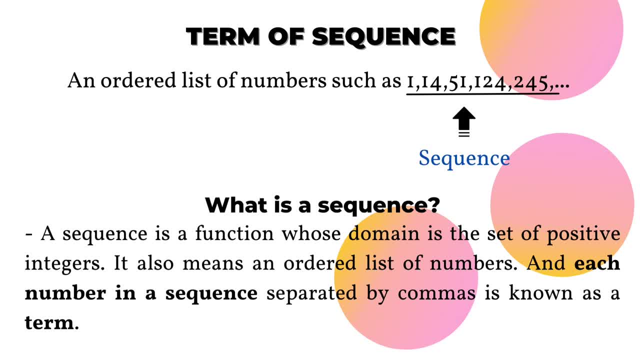 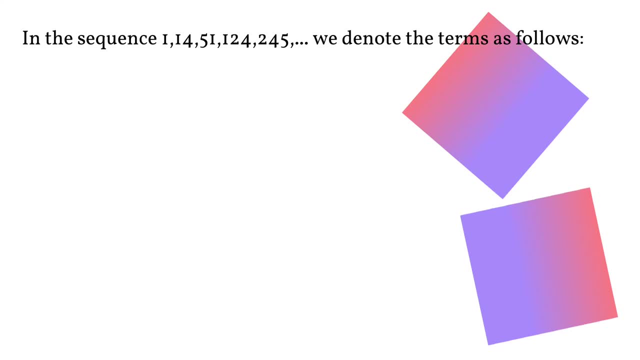 So what is a sequence? A sequence is a function whose domain is the set of positive integers. It also means an ordered list of numbers, And each number in a sequence separated by commas is known as a term. So in the sequence 1,, 14,, 51,, 124, and 245, we denote the terms as follows: 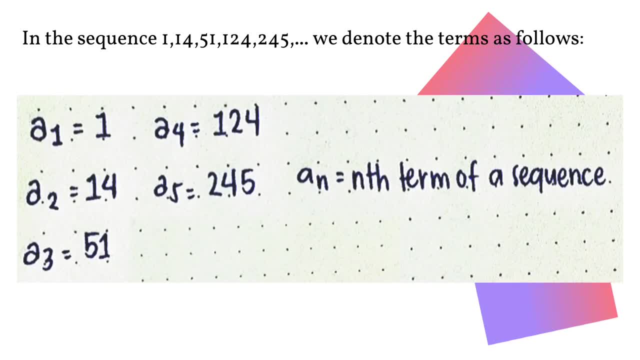 So a sub 1 is 1, since that is our first term. a sub 2 is 14, since ito yung ating pang second term. The next is a sub 3 is 51, since that is our third term. a sub 4 is 124, dahil yun ay ating pang apat na term. 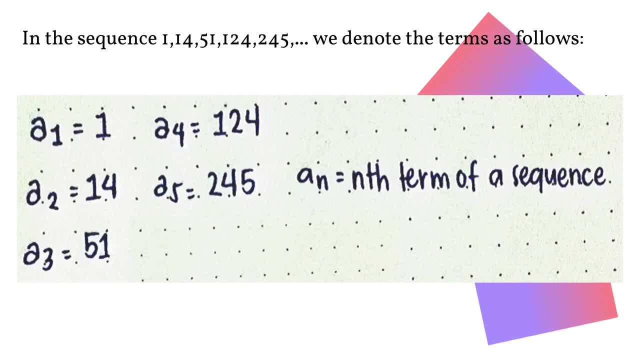 Then next ulit ay a sub 5.. The last one is 245, dahil yun ang ating pang limang term, So we simply call this a sub. n is the nth term of a. If you notice, there is an ellipsis at the end of our sequence right. 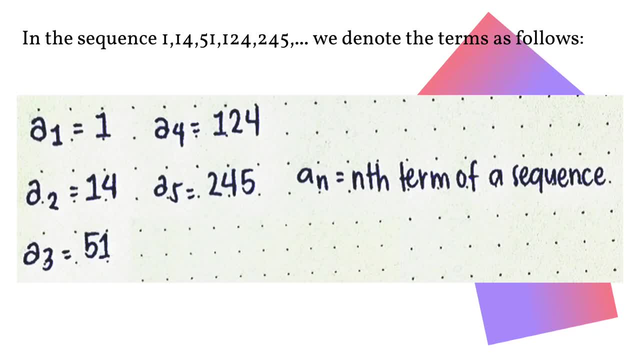 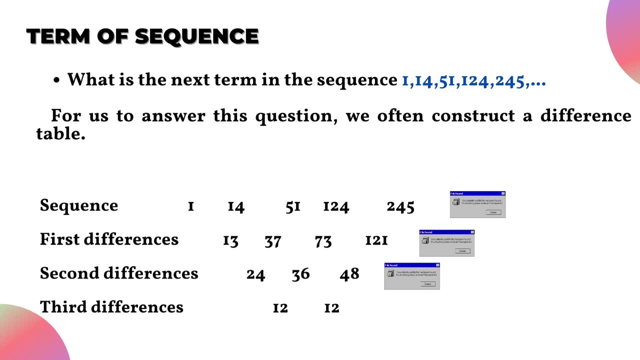 So, for you to know, yung tatlong tuldok, dyan o ellipsis, ay nagpapahihwating na the sequence continues beyond 245.. So para mas maintindihan mo, let's have this example. So what is the next term in the sequence 1,, 14,, 51,, 124, and 245?? 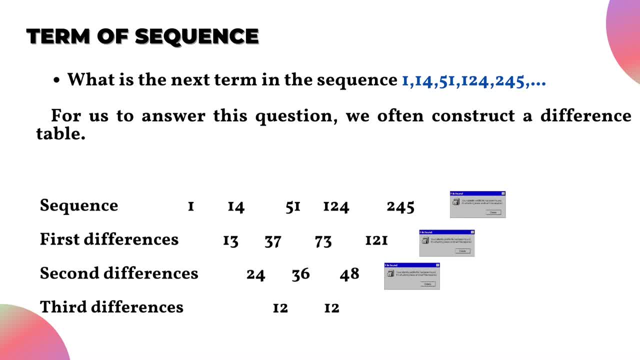 Bale, para makuha ko yung sagot, ginamit ko yung difference table, which is a method na madalas ginagamit when it comes to finding the next term of a sequence. Kaya, sa pamamagitan ng paggamit ko rito ng sequence, makukuha ko yung differences ng bawat term, kung saan, if mag-i-equal na siya. 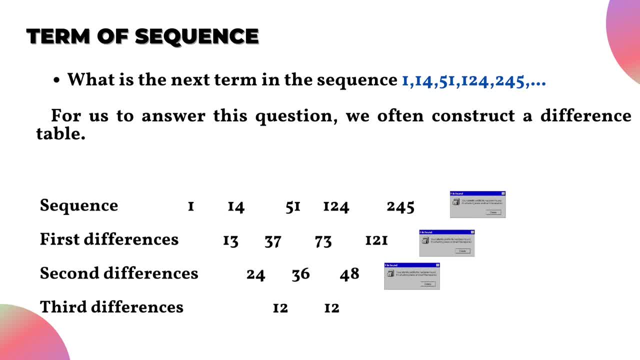 malalaman ko na kung ano yung next term, which is what I am aiming to obtain Now, paano ko ba nagawa yun? Una, kinuha ko yung first differences nila, so ginawa ko yun by subtracting the first term sa second term. 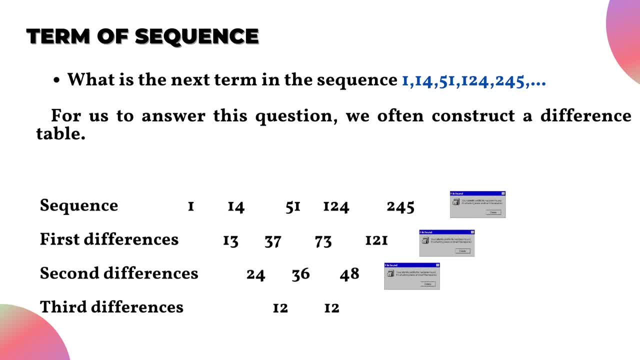 So 14 minus 1 is equals to 13.. 51 minus 14 is equals to 37.. 124 minus 51 is equals to 73. And 245?? 245 minus 124 is equals to 121.. Ayan, hindi pa rin siya equal. 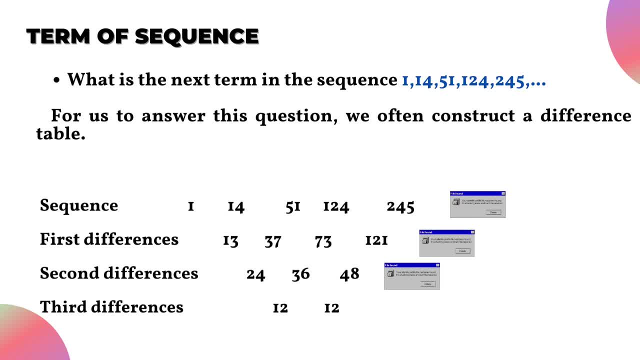 So sinubukan ko naman kunin yung second differences nila, and still hindi pa rin equal. So hanggang sa umabot na ako sa third differences at at this time nakuha ko na yung differences nila, which is 12.. 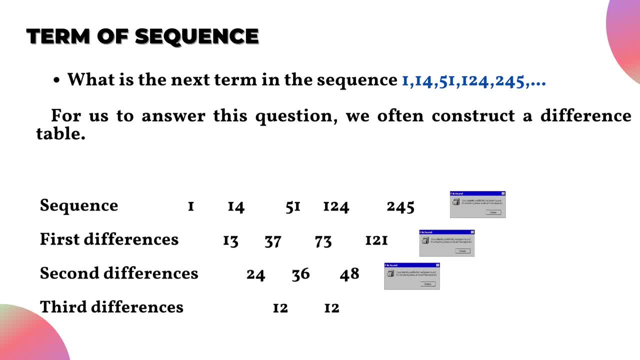 So paano ko naman nakuha yung next term sa second differences. So bale, kung mapapansin mo, pag minus ko yung 48 sa 12, ang sagot niya is 36.. At kapag in-add ko naman yung 36 at 12, ang sagot niya is 48.. 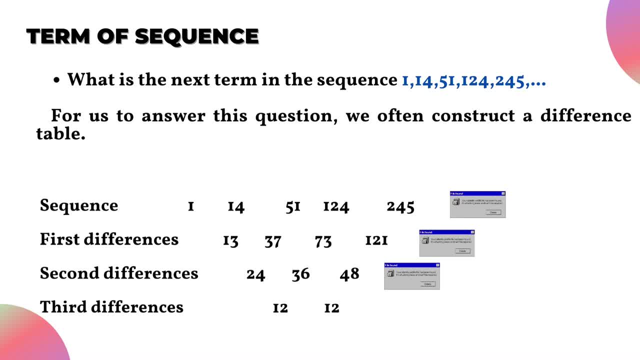 Ang gagawin mo lang is i-add mo yung 48 sa 12 and that is equals to 60.. Which is yun na yung next term ng ating second differences. Bale, ganoon na rin yung gagawin natin sa next. 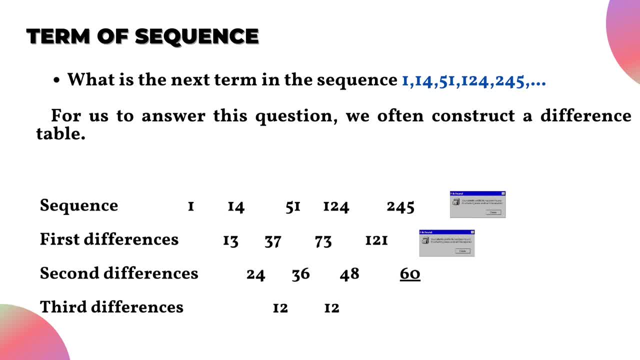 So i-add natin yung 60 sa last term ng first differences. So 121 plus 60 is equals to 181.. So para naman makuha na natin yung next term ng sequence na mismo, add natin yung last term ng first differences sa last term ng sequence. 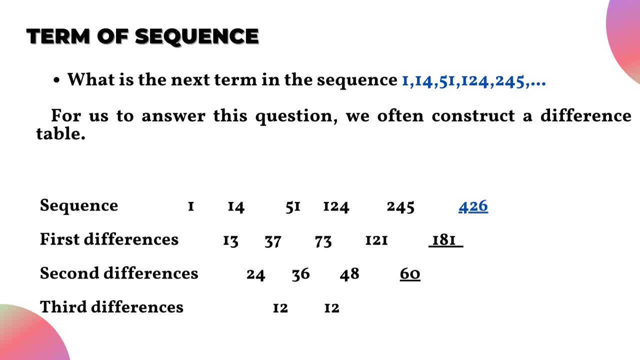 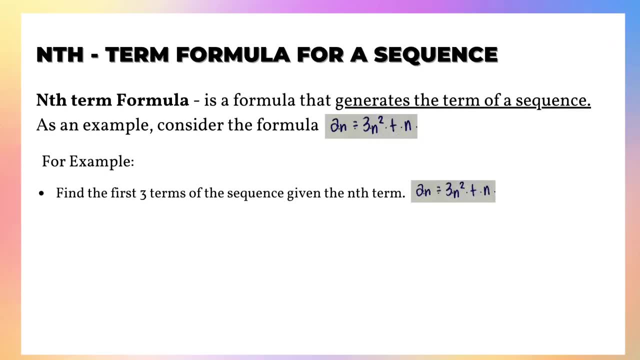 So that is 426.. So therefore our next term sa sequence is 426.. So in our previous example gumamit tayo ng difference table para malaman natin yung next term ng isang sequence. Pero sa ibang cases pwede tayong gumamit ng pattern sa pagpindik ng formula. 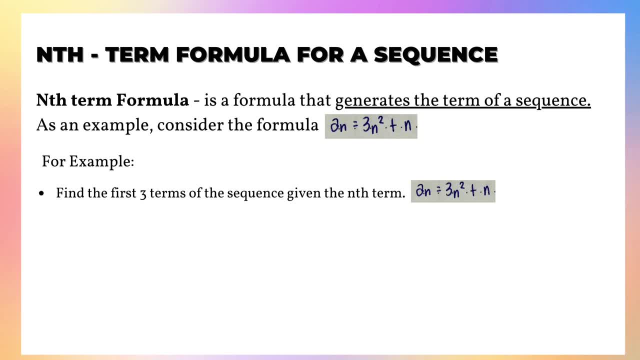 And that is what we refer as nth-term formula. Nth-term formula is a formula that generates the term of a sequence. As an example, consider the formula: a sub n is equals to 3n squared plus n. So let us have this example. 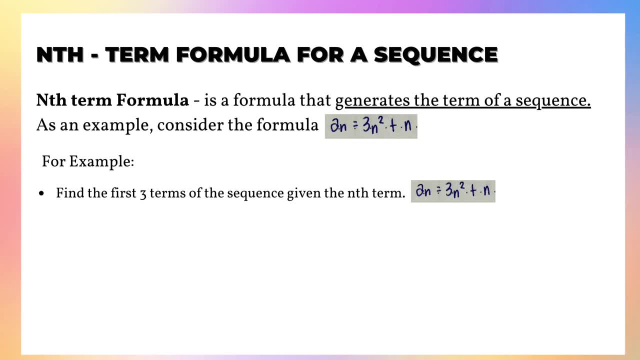 Find the three terms of the sequence Given the nth term. So, in finding the answer, susundan natin yung rule or formula a sub 1,, since we denote that as our first term, and papalitan lang natin yung n ng 1,. 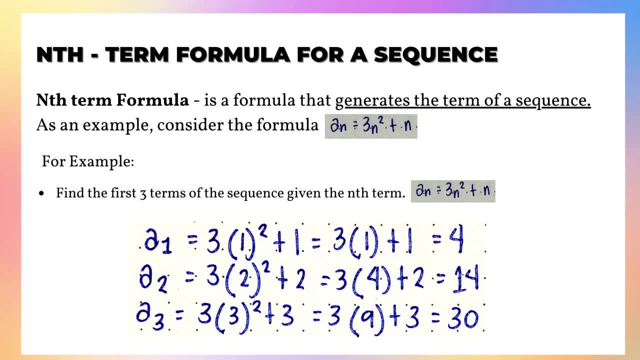 kaya for that reason magiging 3 times 1, squared plus 1 na siya Kaya naging 3 times 1. siya kasi diba yung 1 natin may squared. So 1 times 1 equals 1.. 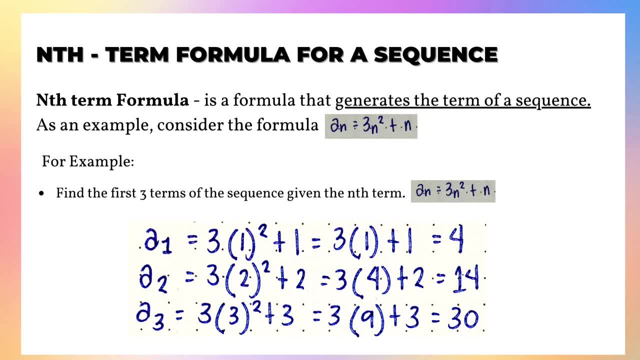 3 times 1 plus 1 is equals to 4.. And that is our first term. Now sa pagkuhan natin ng second term and third term, ganun lang din yung susundan natin na procedure. So our first three terms of the sequence, given the nth term, are 4,, 14, and 30. 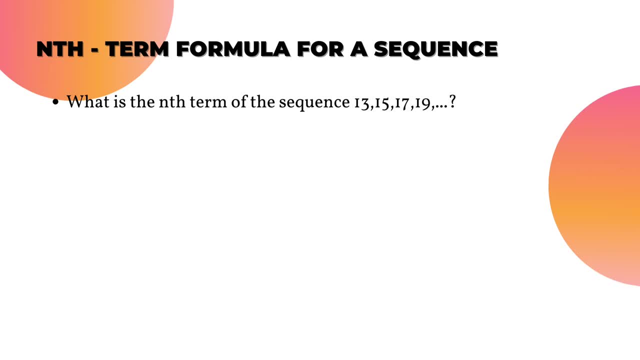 What is the nth term of the sequence? 13,, 15,, 17,, 19?? Bale sa previous slide natin provided yung nth term. Tapos ngayon, paano natin nakukuha yung sagot if sequence lang yung given? 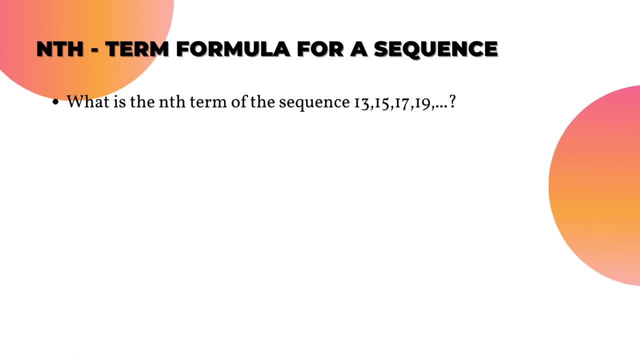 So, given the sequence, kukuni natin yung sagot by using the general rule for nth term, which is madalas kinagamit. Ngayon kukuni natin yung first term. So substitute natin yung a sub 1 at yung n natin, which stands for 1.. 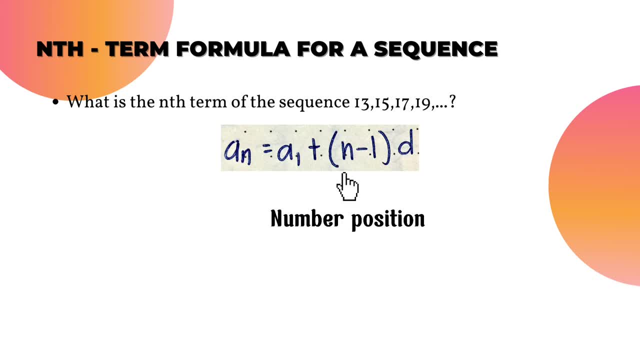 At yung n natin, which stands for number position in a given sequence, At yung di naman dyan sa formula, depicts for the common difference. So when we say common difference, yun yung kapag sinasubtract natin yung mga terms, 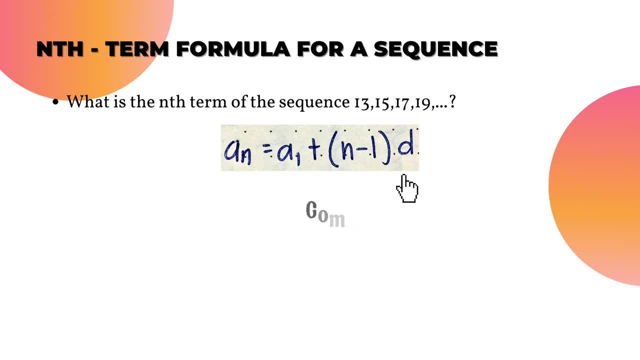 and kinukuha natin yung difference nila na same ng value, So a sub 1 is 13, since yun yung ating first term. Then common difference naman nila ay 2.. And I know alam nyo nakunin yun, kasi natakal na natin yung kanina. 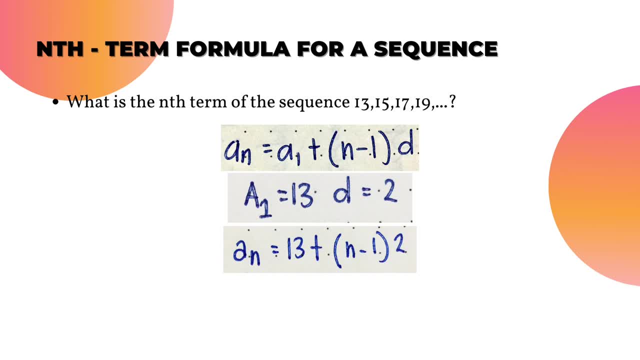 Ayan, substitute na natin, And that is a sub. n is equal to 13 plus n minus 1.. And common difference naman ay 2.. After that, simplify na natin. So, by using distributive property, mamultiply natin yung 2 sa n and negative 1.. 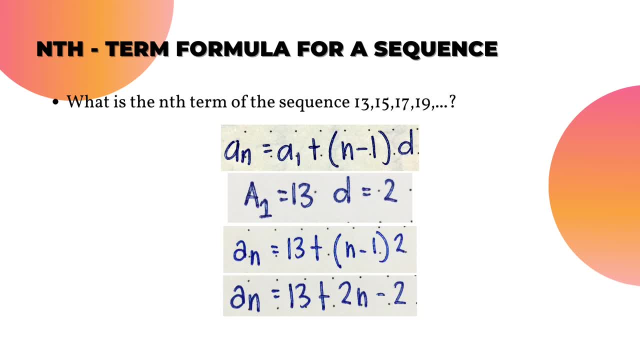 So 2 times n is equal to 2n And 2 times negative 1 is equal to negative 2.. Let's combine similar terms, As what you can see: walang kapareha si 2n, So kukopihan lang natin sya. 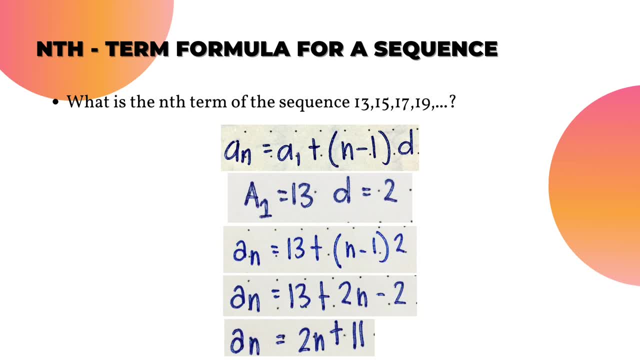 Then yung dalawang value natin na natila pagsasamayan natin. So 13 minus 2 is 11.. Thus the nth term of the sequence, 13,, 15,, 17, and 19 is 2n plus 11.. 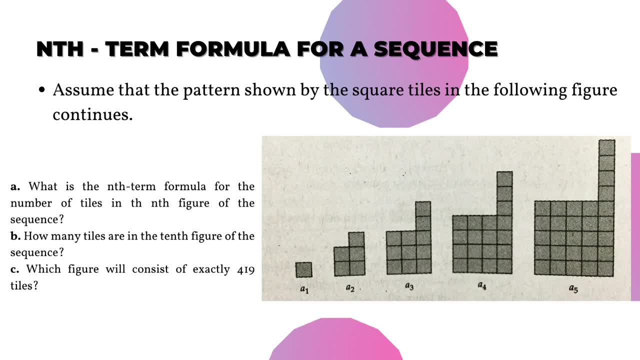 Let us have another example. So assume that the pattern shown by the square tiles in the following figure continues: A- what is the nth term formula for the number of tiles in the nth term figure of the sequence? B- how many tiles are in the 10th figure of the sequence? 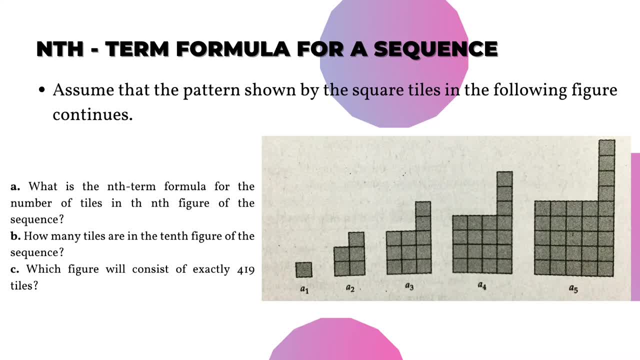 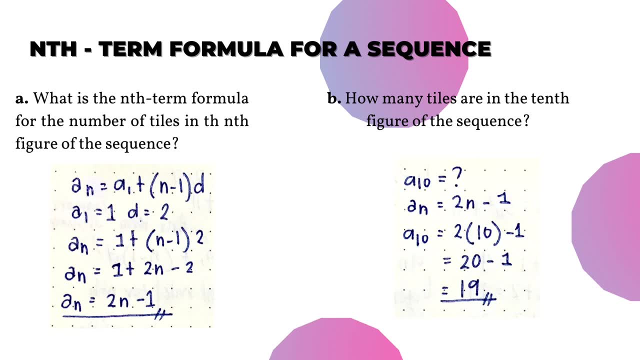 C, which figure will consist of exactly 419 tiles. So sa next slide sasagutan natin yan Bale, pakasettle lang po yung previous slide, kasi andun po yung mga figures at para mas maintindihan nyo po kung ano po yung sinasabi ko. 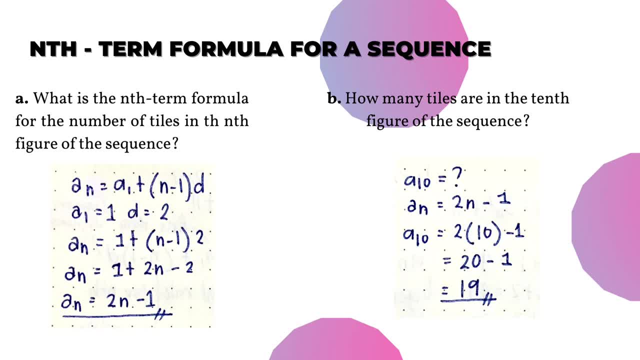 So, observing the figures doon sa ating previous slide, makikita natin na yung ating first term meron syang 1 tile, and sa second term meron tayong 5 tiles, And sa a sub 3 meron tayong 11 tiles, and sa a sub 4 naman meron tayong 19 tiles, and sa a sub 5 naman ay meron tayong 29 tiles. 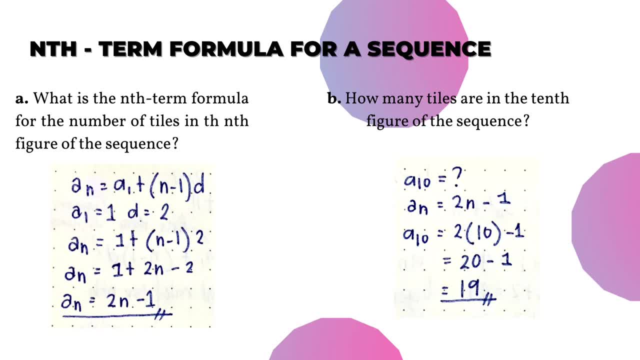 Kaya na-explain ko na yung sagot ko sa A Bale. ayun hinanap ko yung nth term, or pattern that is shown by the square tile, by using the formula na ginamit natin earlier. So ayun kinuha ko yung first term, and that is 1.. 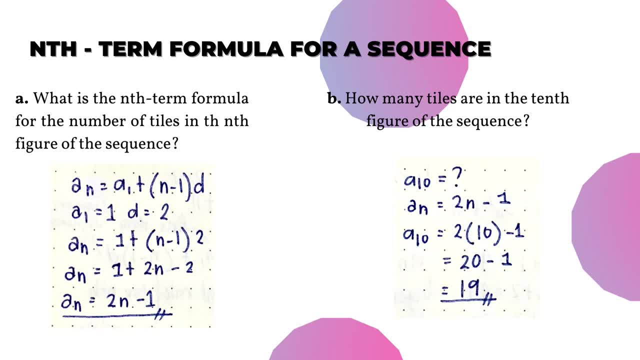 And yung common difference naman nila nakuha ko na kanina and that is 2.. Next step is nag-substitute ako, So our a sub 1 is 1 plus n minus 1 and common difference na 2.. 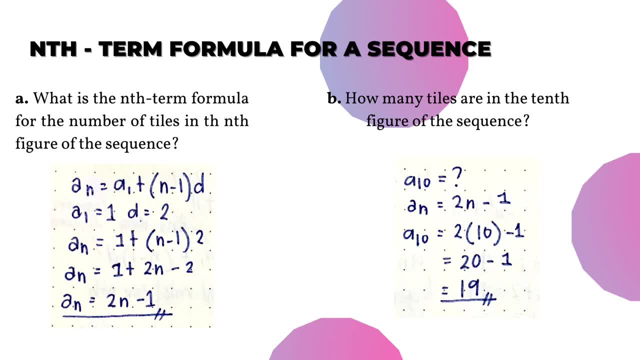 Then distribute yung 2 sa n minus 1.. So 2 times n is 2n and 2 times negative 1 is negative 2.. So, since wala namang kapares yung 2n, kukopyahin na lang natin sya or kinopya ko na lang sya. 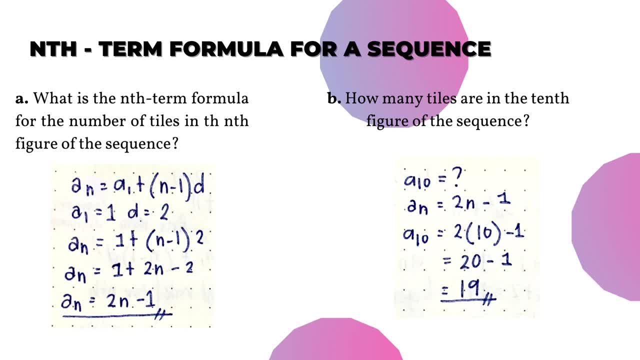 And simplify yung dalawang natirang value. So 1 minus 2 is negative 1.. So therefore ang nth term dito is 2n minus 1.. So sabihin naman tayo: By using the nth term, we can obtain the tenth figure of the sequence. 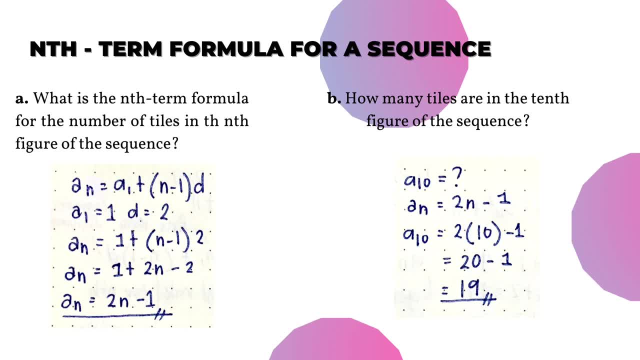 Bale, ito yung ginawa ko first is sinubstitute ko yung given na nth term, So 2n minus 1, papalitan lang natin yung n ng 10.. Kaya 10 times 2 is 20.. 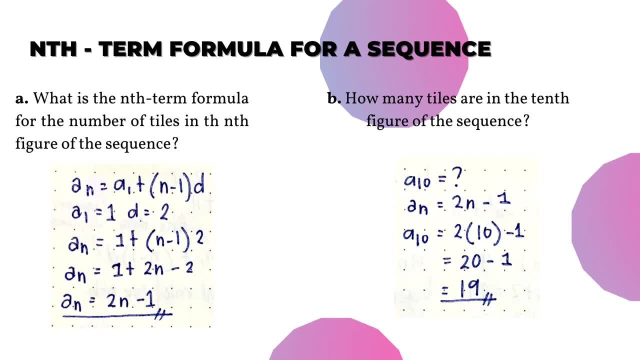 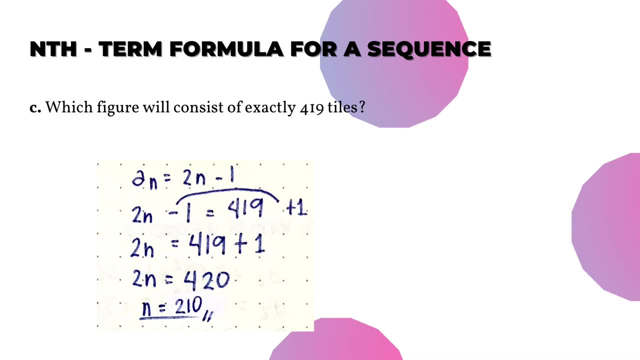 Then minus 1, that is 19.. Thus the tenth figure has 19 square tiles. So nasa C na tayo. So again ginamit ko na naman yung nth term, Kaya by the use of this we will find out the exact position of the n or the position ng figure na may 419 na tiles. 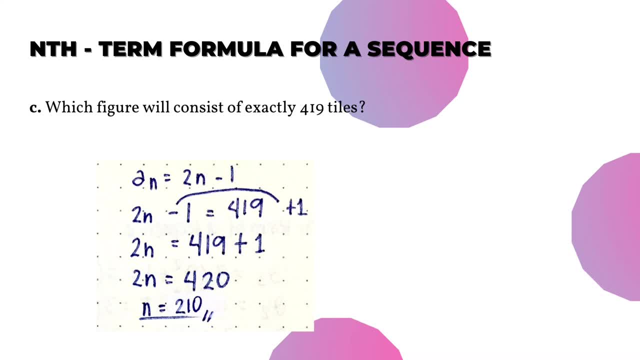 Okay, so 2n minus 1.. So dito ang value daw ng a sub n is 419.. So 2n minus 1 is equals to 419.. And as what you can see, I transpose ko yung negative 1, so naging positive na sya. 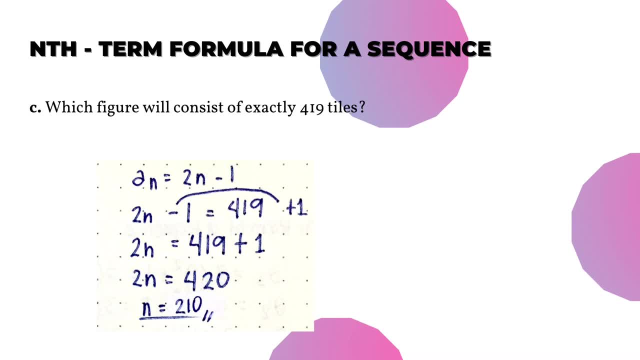 419 plus 1 is 420.. So 2n is equals to 420 and divide ko yun by both sides And the result is yung a sub n is 419.. And the result is yung n, or figure na yun ay pang 210.. 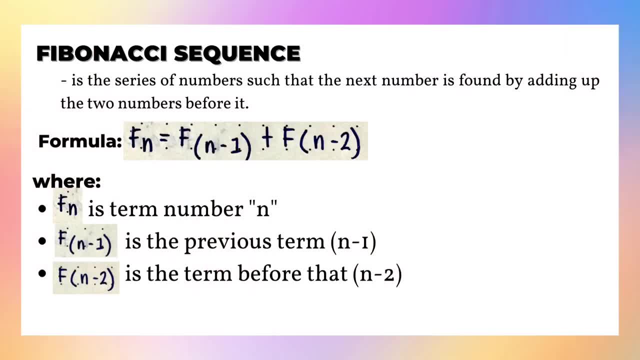 Let's proceed. So Fibonacci sequence is the series of numbers, such that the next number is found by adding up the two numbers before it. So here we can make use of this formula: F sub n is equal to F sub n minus 1 plus F sub n minus 2.. 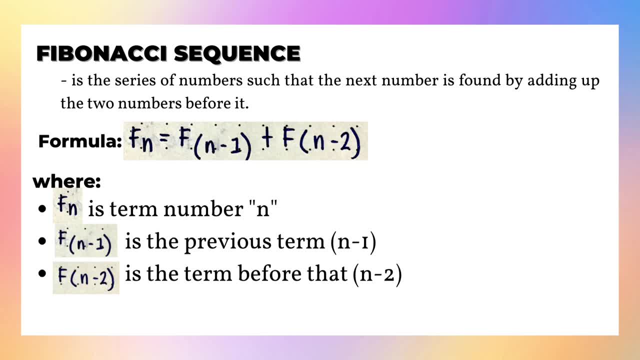 Where F sub n is term number n or the number position in a given term, And F sub n minus 1 is the previous term, or n minus 1.. And the F sub n minus 2 is the term before that, or n minus 2.. 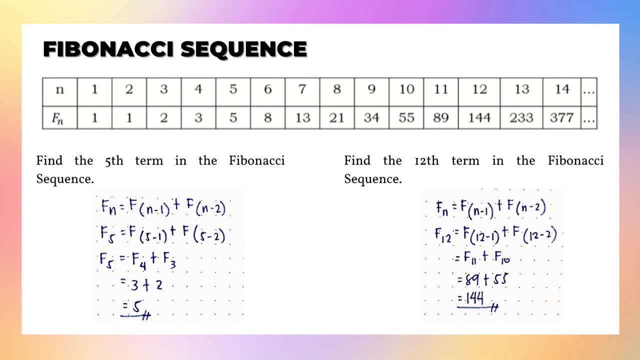 So yung naka-table, ayan yung first 14 terms sa Fibonacci sequence, And ayan sa baba ng table. madalawa tayong examples, dyan, and I will be explaining it. Okay, so find the fifth term in the Fibonacci sequence. 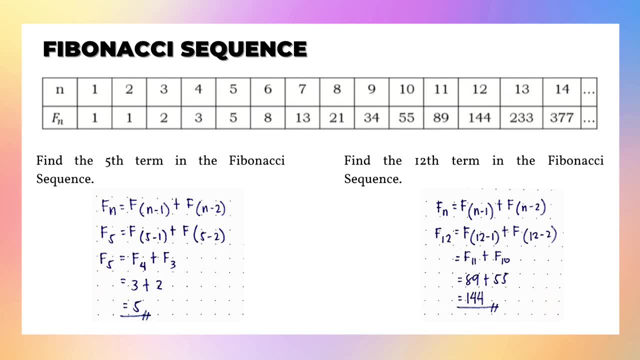 So by using our formula, pinalitan ko lang yung n ng 5.. So magiging 5 minus 1 na yung nasa unang, naka-enclosed sa parenthesis and sa pangalawa naman magiging 5 minus 2 na sya. 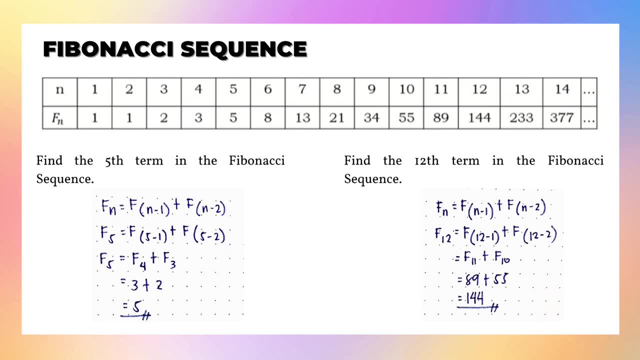 So kukunin natin yung F sub 4 sa table and that is 3, kasi yun yung value nya, And yung F sub 3 naman is 2.. So 3 plus 2 is 5, which means yung F sub 5 natin is equals to 5, which is tama. 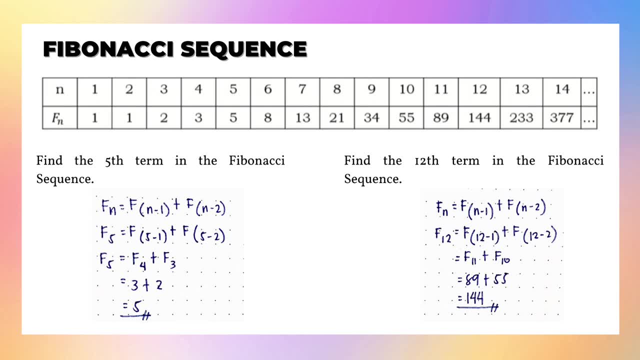 Sa pangalawang example same method and formula, lang din yung ginamit natin. So yung n pinalitan lang natin ng 12 and then mininus natin yung mga value na naka-enclosed sa parenthesis. 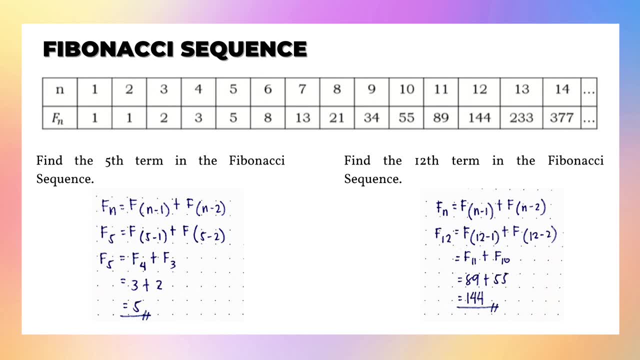 And then hinanap natin yung F sub 11 and F sub 10.. Then pinag-add natin yung value nila and that is 144, which is correct also, Kasi makikita mo sa table na yung F sub 12 ay may 144 na value. 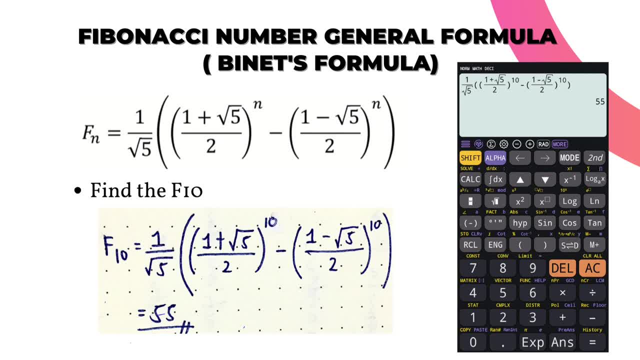 Aside dyan, there is a simpler way, and that is by using a calculator and a formula to easily obtain the answer without having the table. So that formula is called the Fibonacci number general formula or Binet's formula, which is a formula that incorporated the golden ratio. 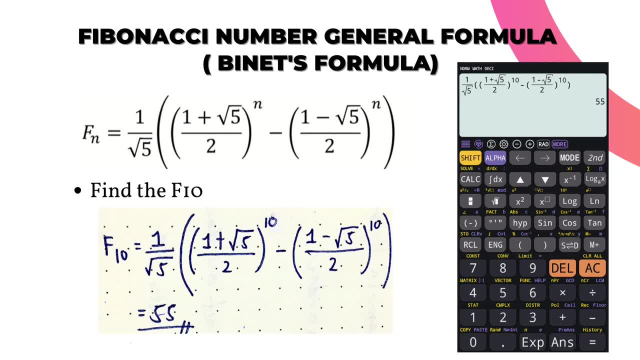 So in here F sub n symbolizes the nth term. The nth term where F sub n is equal to 1 over square root of 5 times the quantity of 1 plus square root of 5 over 2 raised to n minus 1.. 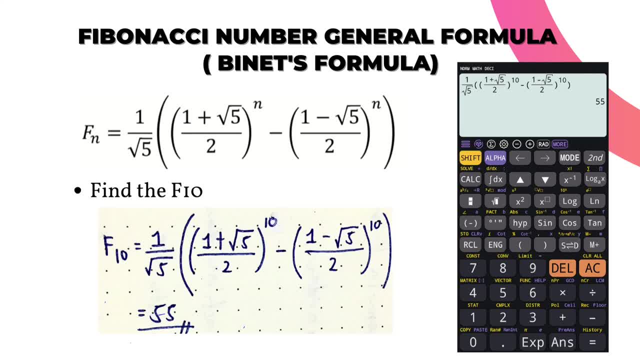 Minus square root of 5 over 2 raised to n. So dito, papalitan lang natin yung n ng 10, as easy as that, and itatype mo yan sa calculator And tsaraan, may sagot ka na agad. 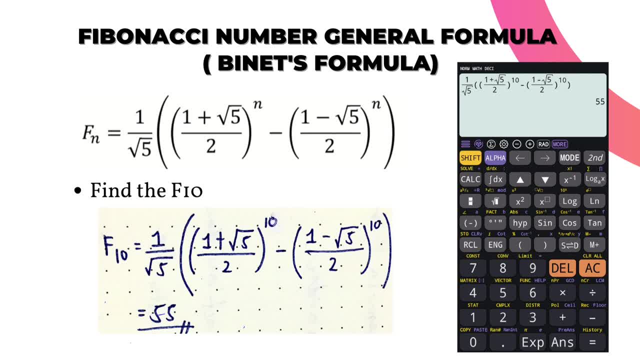 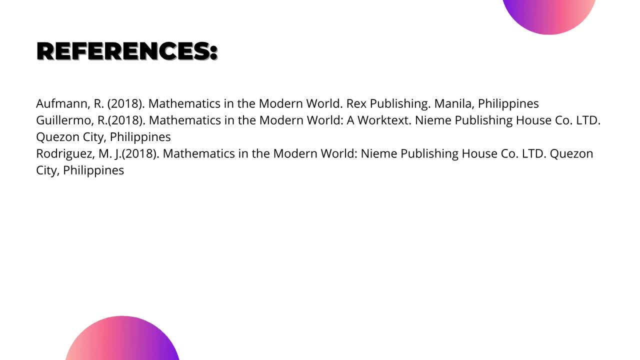 Kaya if nagmamadali ka. this is the best formula that you can use: Siyempre by using a calculator. Special thanks to Wowmat for serving us today. He was my guide in making this video. Okay, we're done. Thank you for watching and I hope you learned something today.